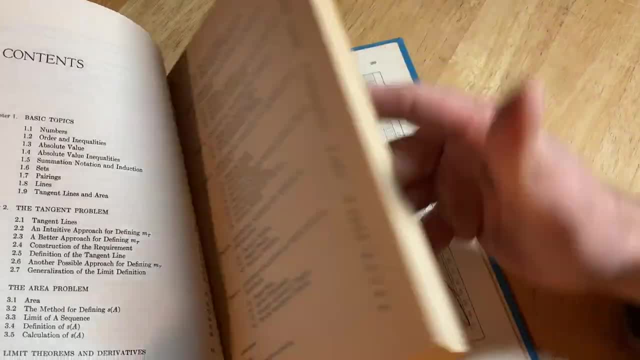 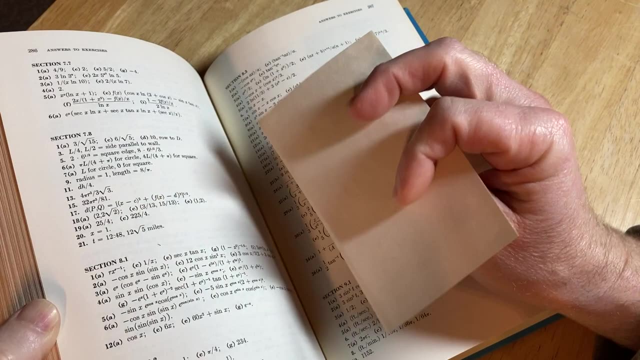 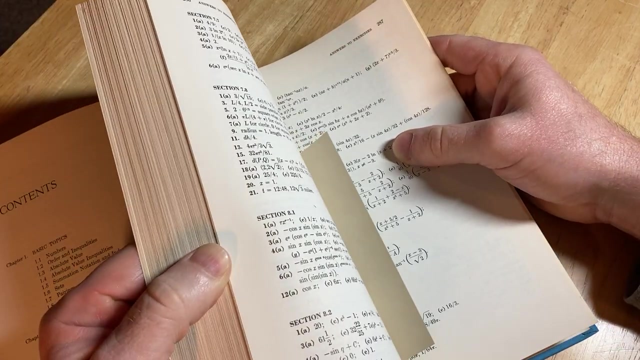 stuff that is not here. So let's look at the answers, Page 277.. There's a little card here. It'll leave it up there. I feel like it came with the book. It should be preserved. Yeah, it looks like you have answers to some of the exercises, not all of them. That's pretty. 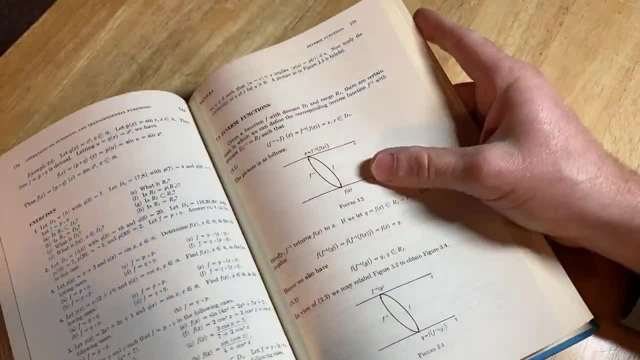 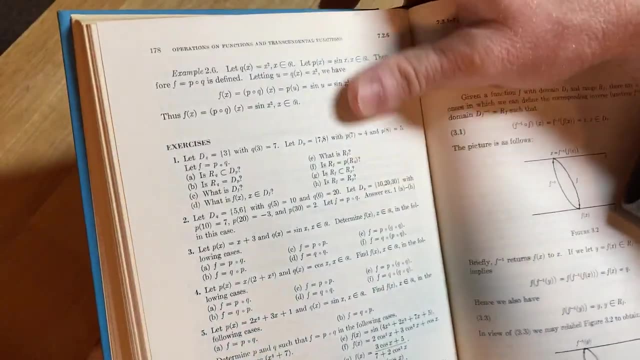 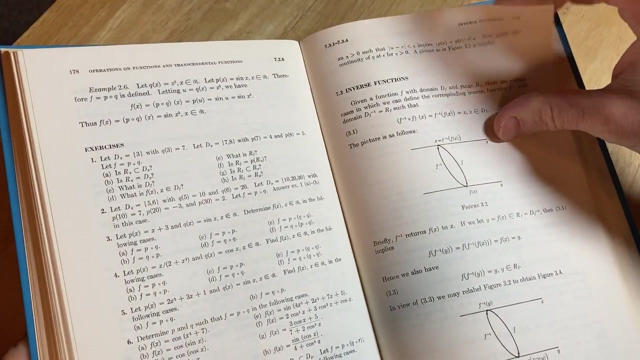 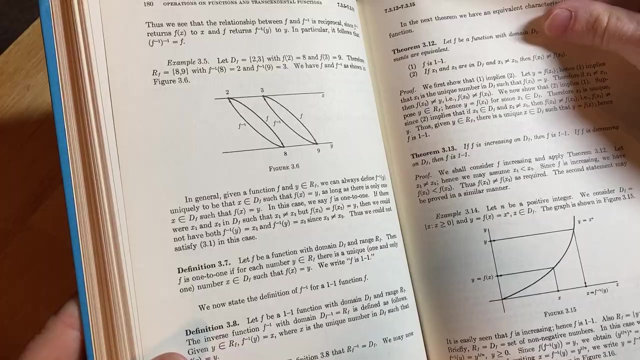 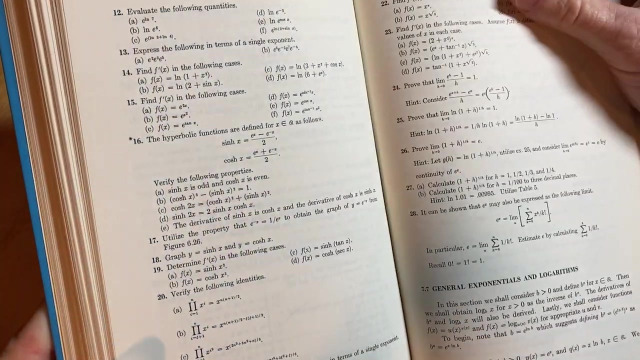 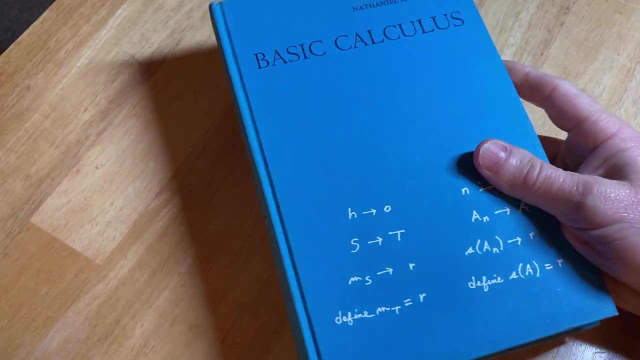 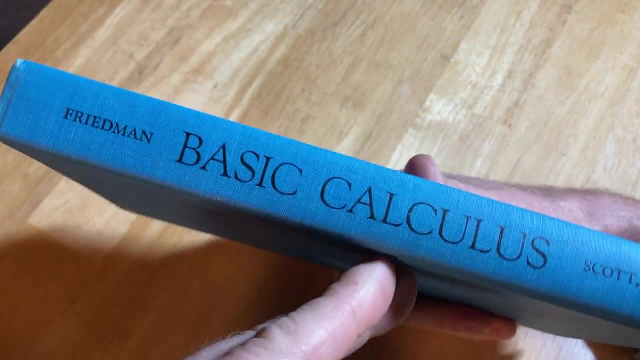 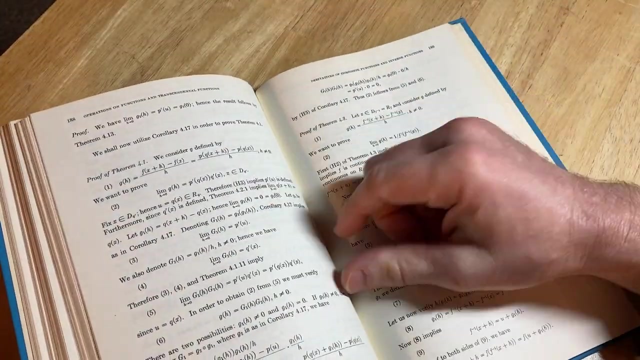 It's really blue. I don't know if it's really coming out in the camera, but it's shockingly blue. It's a very, very, at least this particular edition. If I can find the copy, I'll leave a link of some edition in the description of this video. I don't know if this book is. 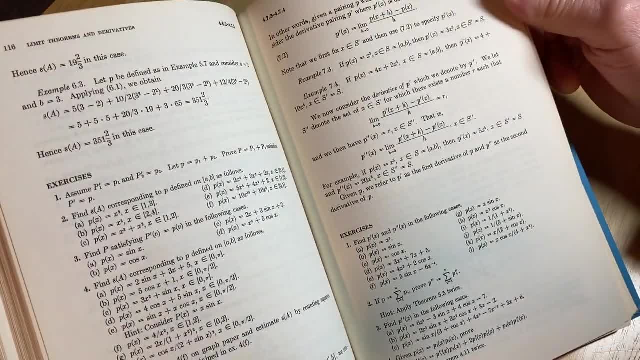 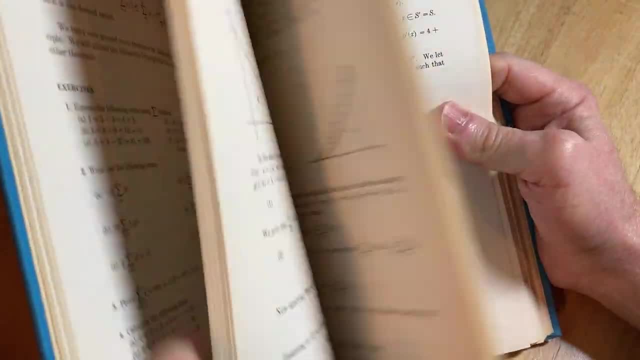 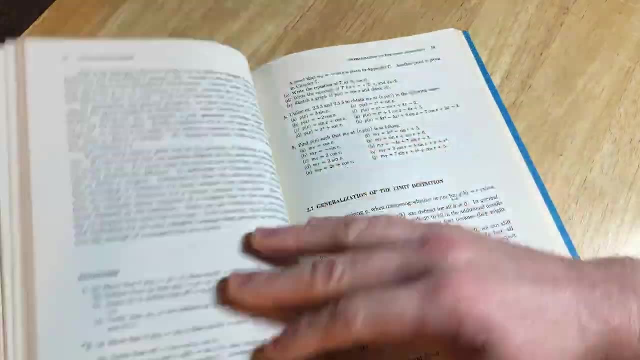 still in print or anything. but yeah, interesting, Find some derivatives here. It's pretty easy. Most of the mathematics seems it's basic calculus. but old books like this, they do give you a different perspective. The explanations are different. You know, reading someone's. 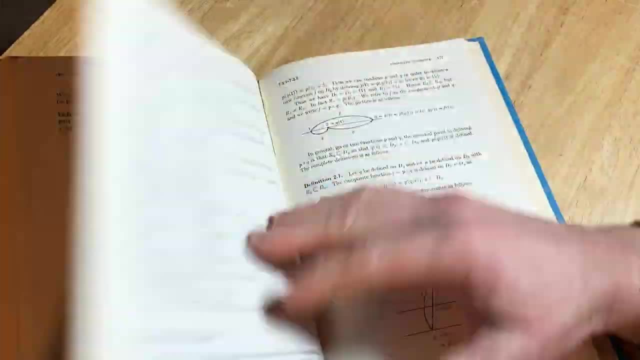 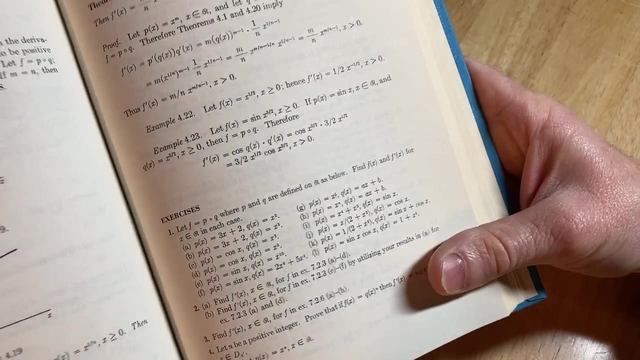 take on something, or just seeing it again, it's like: oh yeah, you know, I think it helps solidify ideas. So yeah, Just wanted to show you this book. Keep doing math. 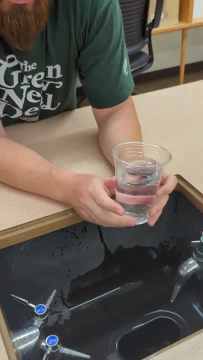 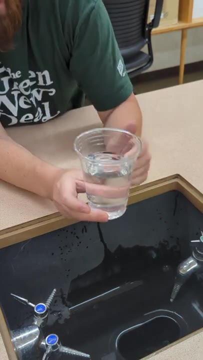 If you ever dove into a pool, you would feel that the deeper you go, the higher the pressure is in the liquid, And that really comes down to the fact that the pressure at any depth in the liquid depends on all the liquid above it.